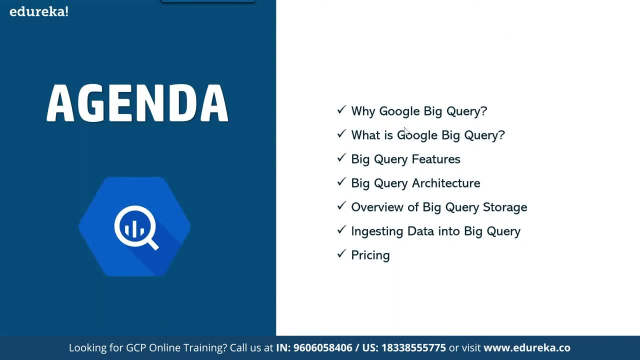 What exactly is cloud computing? What is GCP? We'll talk about. why Google BigQuery? What exactly is Google BigQuery? Some of the features of BigQuery, its architecture, the overview of BigQuery, storage and ingesting data into BigQuery. and the pricing. 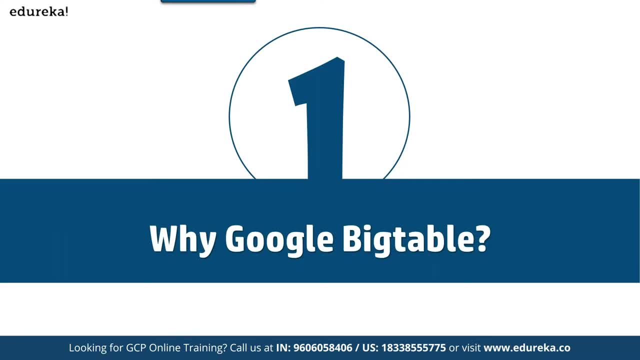 So now let's get started and get understanding. So, what exactly is Google BigQuery? What exactly is Google BigQuery? What exactly is the cloud? You know what exactly is the virtual machine? Virtual machine is basically is the simulation of the computer system. So now, what exactly is GCP? GCP basically stands for Google Cloud. 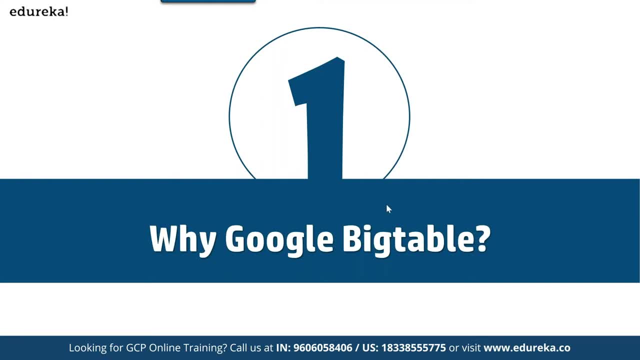 Platform. This is a cloud service which is basically, you know, being provided by Google. So we are in. you know, Google is going to host your entire data on the platform. So you can do everything. You can create a virtual machine, You can create a database- Any kind. 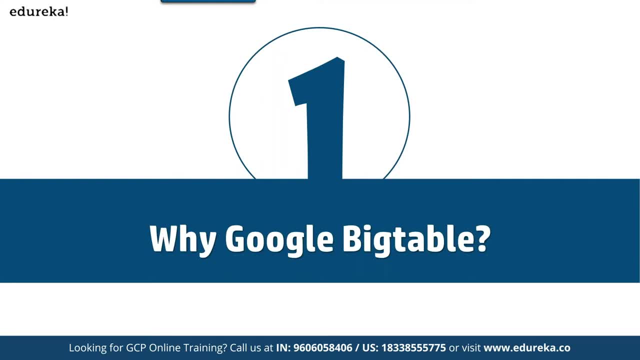 of the things that you can do at your on-premise platform can be done on the cloud at the safe, of ease. At the same time, you can perform that integration with different tools, technologies that Google has very easily. So now let's talk about you know why Google Bigtable Before we talk about you know. 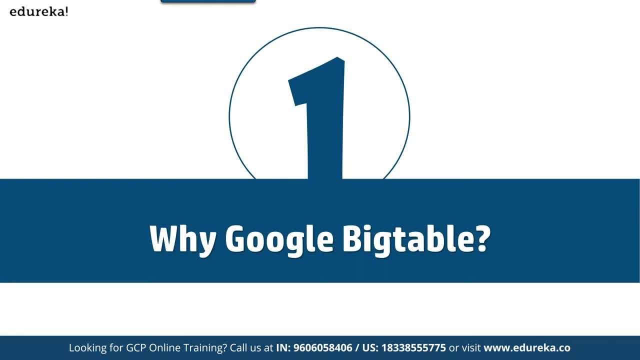 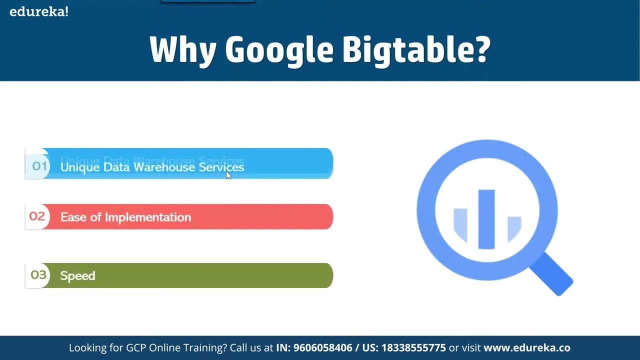 why Google Bigtable? What is the use case of it? Why exactly we should use Google Bigtable? These are a couple of advantages. So it has unique data warehouse services. So your data locations various places, So it has a unique data warehouse services. It's not like that. 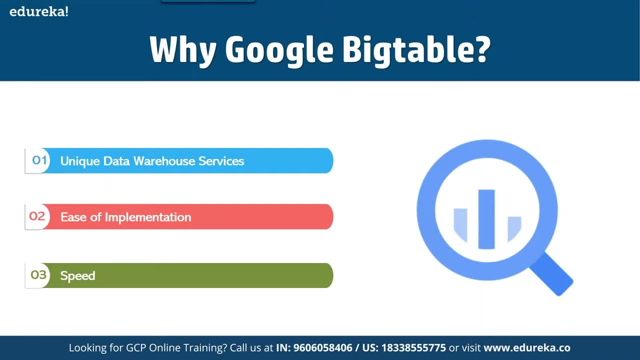 you know, at the same one data center you're accumulating all the data for all the customers, So it basically provide you high availability And at the same time, it has the unique services for each of the user. Second is ease of implementation. to work on This is very easy. Some people. 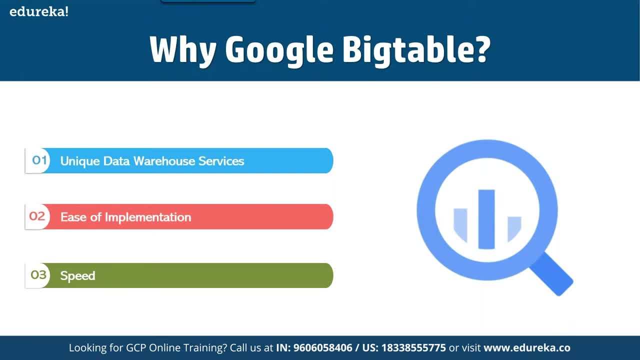 think that, oh, it's a cloud, So it's very difficult for you to use and implement. We have to. you know, say we get a network, It's going to be very complex. So once you're going to work, you will see the interface You're going to get. 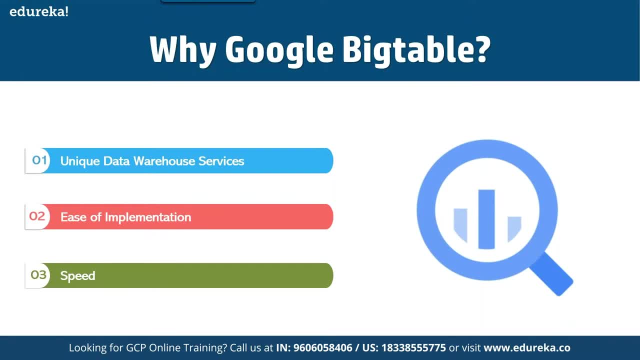 An opportunity to work on this and dive in more detail. You will see it's very easy. Plus the speed, It's very fast. Now, for example, you are going to create the resources. Let me, you know, give you a very small example. I have to install an operating system on my 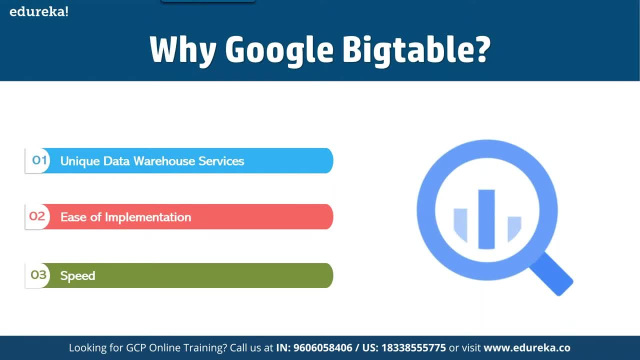 laptop, How much time it takes- Approximately an hour, right. Or if I have to also, let's say, you know, create a virtual machine on my system, it will take how much time, Approximately an hour. Here, in the case of Google GCP platform, you can spin up the resources in, you know. 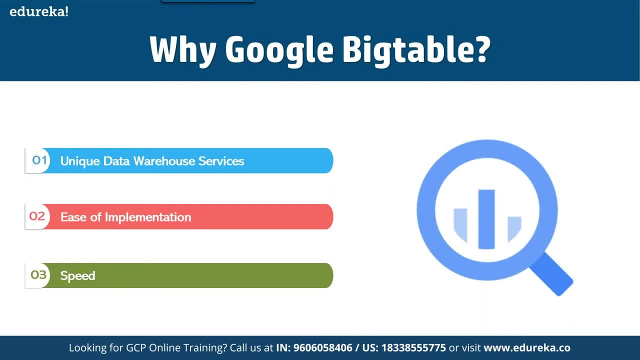 less than five minutes. If I had to create a virtual machine in less than five minutes, I can create it all, And you know it's not going to be an issue. So by the same time, it's going to provide higher availability as well If my data is going to be lost, like 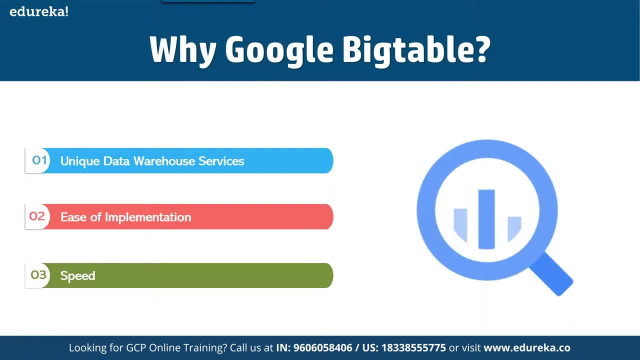 let's say, if my you know where I hosted my data, like in my on-premise environment at my data center. if the data center goes down, my entire data will go down right. However, in this case, that's not the case. If your primary data center is down, it's. 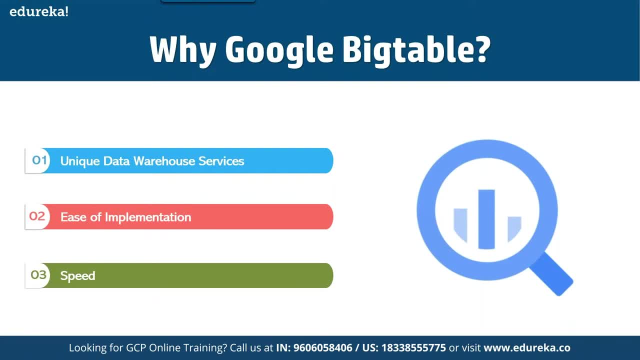 going to perform automatic replication, So data is going to be replicated. So if you don't have a primary data center, you don't have a primary data center, you don't have a primary data center. So you can do it very easily. 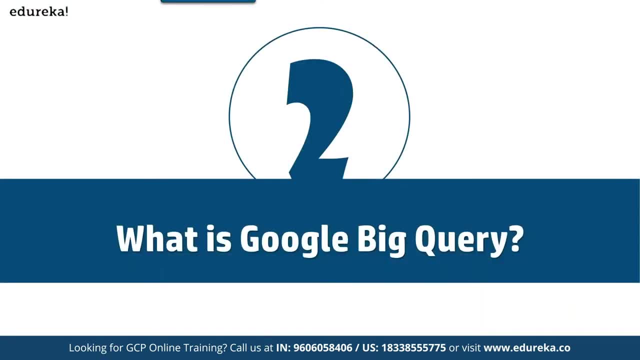 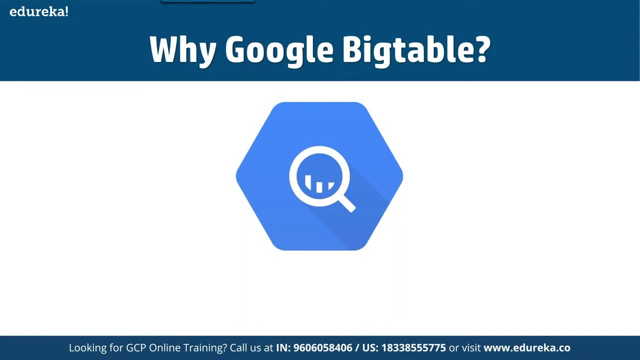 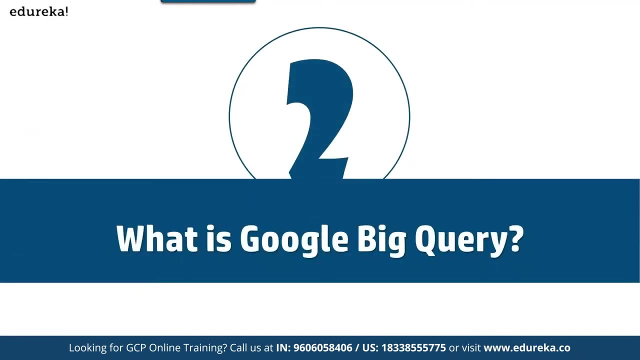 Now, what is Google big query? Let's just get understanding of it. So before that, you know, let's understand Google big table and BigQuery. So basically BigQuery- now you're talking about, you know this guy. So basically BigQuery is a fully managed 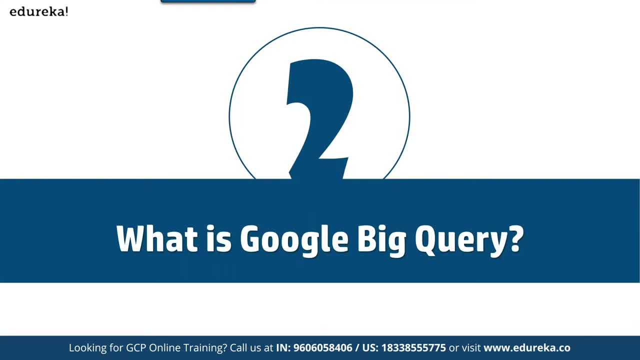 serverless data warehouse service that enables scalable analysis over petabytes of data. So this is a PaaS, which is platform as a service That supports querying using Ansys SQL. So you can, you know, store the data in a large storage and whatever you're going to consume, you're going to pay for it. Now, what are? 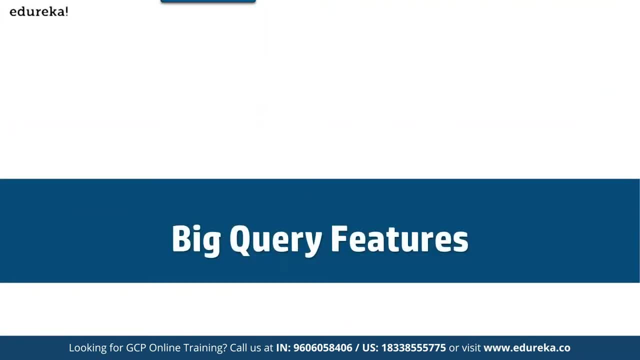 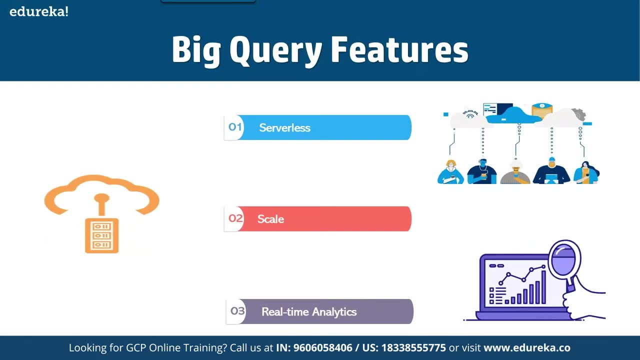 the different features of it. Now, coming to different features, it has various features like: first is serverless. What serverless means? It means that in order to run this, there is no dedicated server required. Now you know that if I had to basically run the 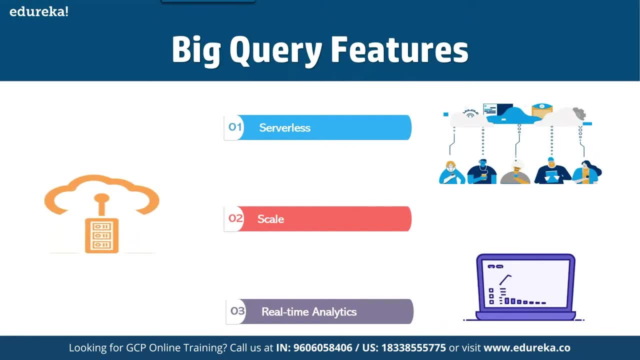 resources. what I will need: A resource, a virtual machine, basically that way that I will require to run those resources, right, So it's a serverless. You don't require the server. without having the server, You basically can, you know, deploy your resources, You can access it, You can integrate with. 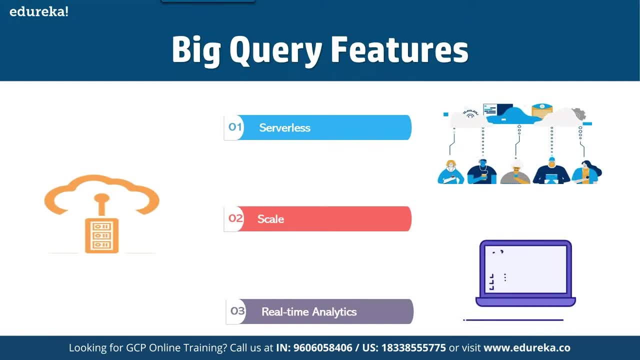 the application Plus, since you are not going to use a server. so having that overhead to manage the server, performing the patching, installing the updates, you know, even paying for that dedicated environment, you can just save the money on that. Second is scale. So 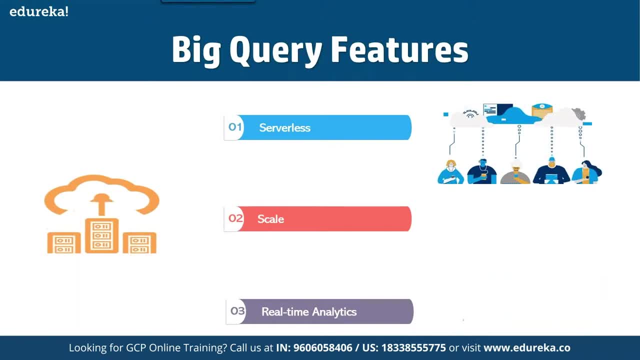 it. basically you can perform the serverless, You can perform scaling as well, You can basically perform automatic scaling. At the same time, you know it's basically supports petabyte of data. So if you want to basically scale with, let's say, you know more CPU, more RAM, that you can do it very easily with this. 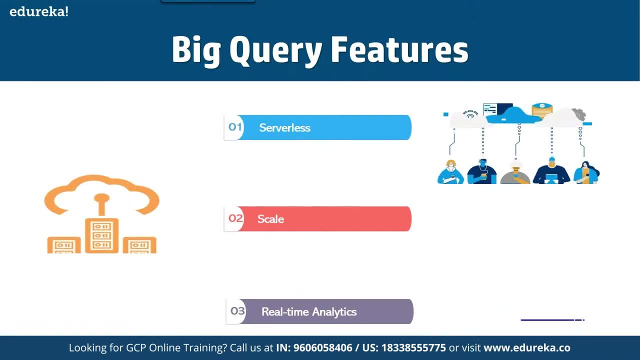 In addition to that, in addition to scaling, let's say, you want to increase number of code processors as well. you can do If you want. you can write the script, you can write the criteria, For example, if your CPU utilization is going to go high at a certain, with a certain 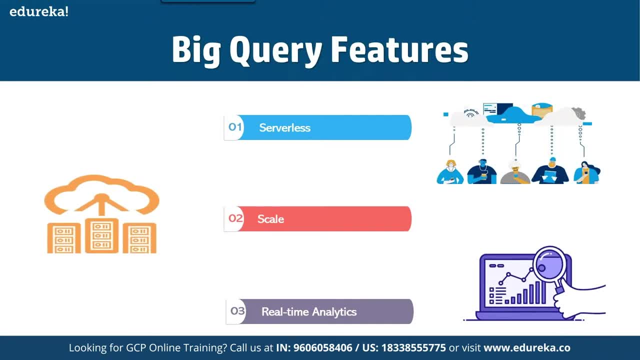 amount. So in this first kind of scenario, what you can do is it's going to automatically increase the resources. When the CPU utilization is going to go low, it's going to automatically decrease the resources. Next is real time analytics, So wherein you can basically inject: 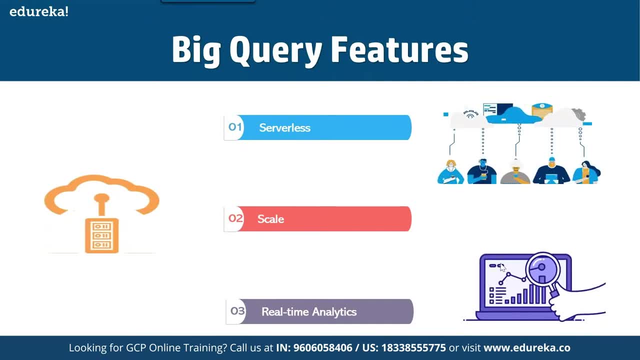 the data from video sources. in this And, as you can see here, towards the right, you can see the progress. Like I want to see my company's going in profit. My company is buying in loss at each and every information at the stake of fees. it's going to be available and you 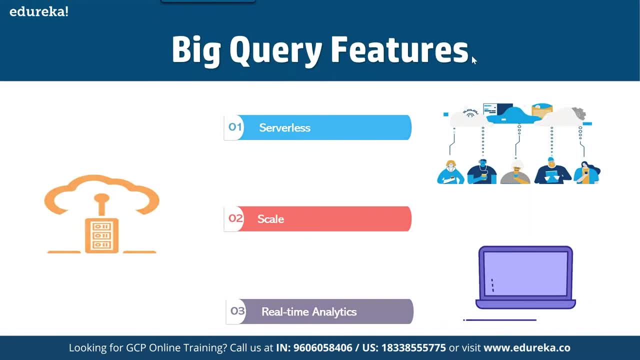 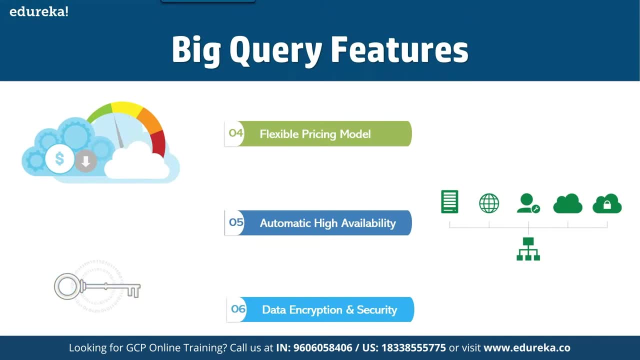 can get that information Very, very quickly. So that's the first kind of scenario. What you can do is it's going to be very easy Now. next one is your flexible pricing model. So it basically provides you various type of pricing model that we are going to dive in more detail today. So it supports flexible 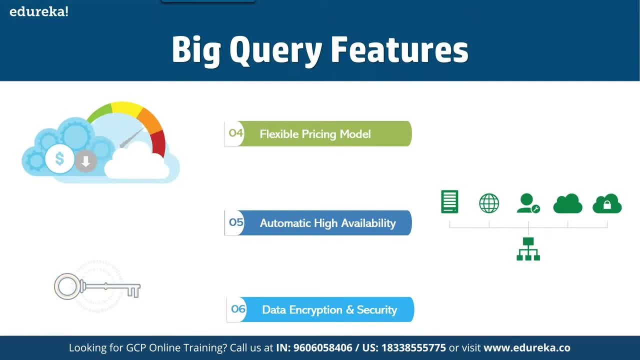 pricing model where you can easily get the. you know, I would say you can easily pick up the package, depending on your need, depending on your requirement. In addition to that, you have to also. you know, you can basically decide that I want. 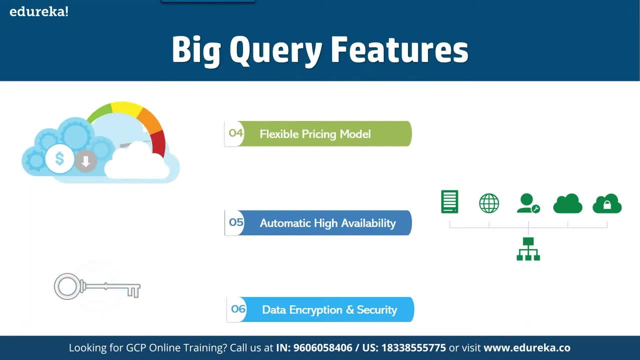 to go with a monthly package, yearly package. I want to go with the services, the way the services I'm going to do, So that's something you'll be able to have that entire. you know flexibility. with this Plus you have automatic high availability. So whenever you're going to create the resources, 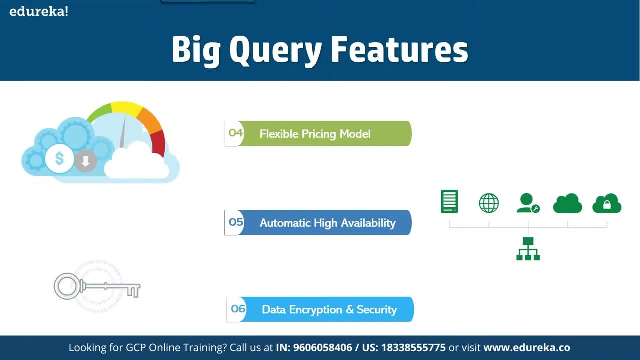 in this case, in the case of bigger Google, BigQuery, those resources, basically, are going to be, you know, replicated at the different sites, depending on the site model that you're going to use. Those resources are going to be, you know, replicated automatically at the same time. 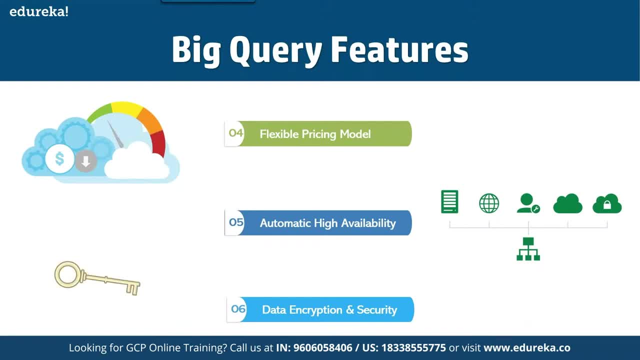 It also supports data encryption and security. So you know that nowadays, encryption is one of the biggest requirement. based on the ongoing hacks, So many companies were hit by the ransomware as well. So in the case of data encryption, what happened is your data is going to be encrypted automatically. 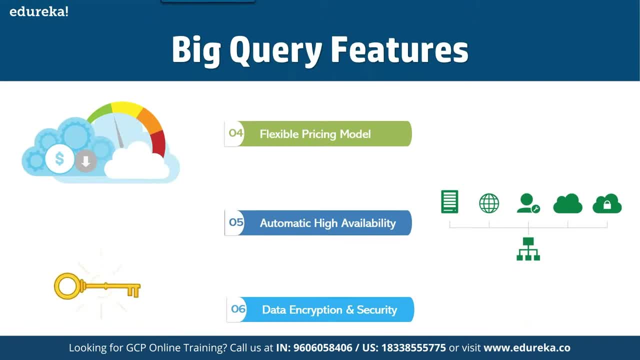 with the key, and that key you can store in a keyword in an HSM, depending on the requirement that you have. So that also provides- and now if I talk about the security it basically supports. you know RBAC as well, which is role based access, wherein you can basically define that you. 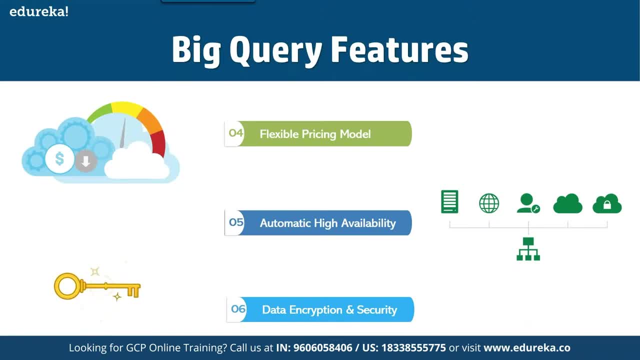 know like which user, which, what kind of role you want to assign. So all this, those are the things that you can do. All those things, basically, are available here as well, at the sake of this. plus, there's no, you know, specific, complex implementation. 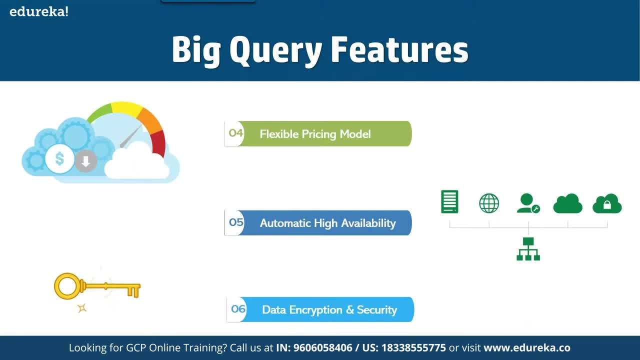 Each and everything is designed in such a way that you can get you know easy interface with easy integrations as well. You can make a API call using different programming languages like Java, Python. different APIs are also available. You just have to change the. you know some variables over there and you will be able. 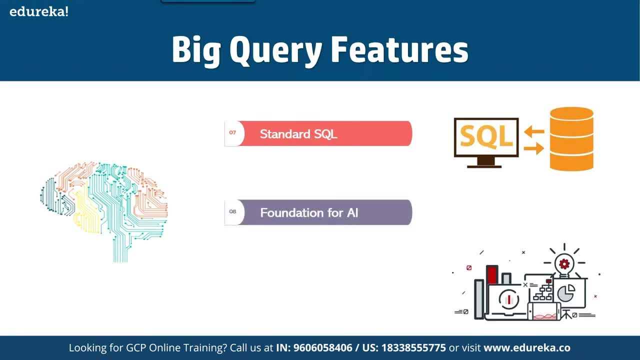 to use it directly. Next one is standard SQL. You automatically have inbuilt standard SQL. at the same time, You can also, you know- define your own database by, you know, creating a new resource, in that you can also create your own database as well. 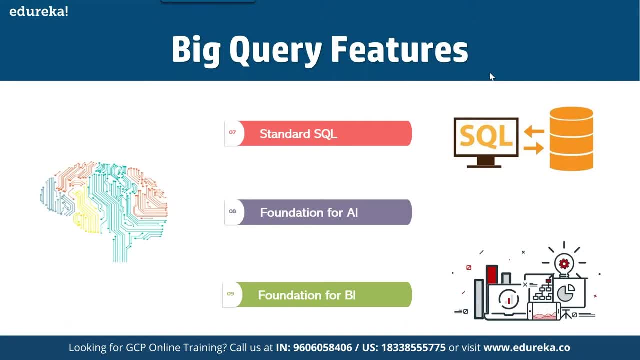 Next is foundation of AI, which is artificial intelligence. You can integrate with- you know artificial intelligence as well- And you can also integrate with DIA as well, which is business intelligence. Yeah, Now, moving on, let's talk about the BigQuery storage. 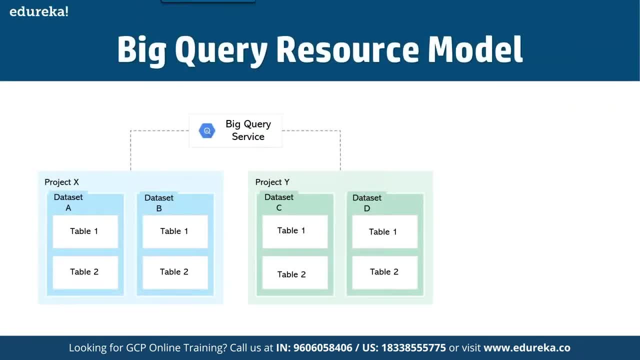 So, in the case of BigQuery storage, It basically has five major components: the projects, the dataset, your tables, your views and the jobs. Now here, in this case, let me just use this highlighter. You know, this is a project, basically one project. it's boundary. 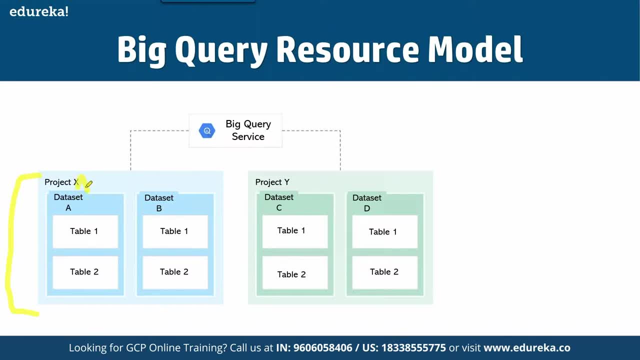 In that project, basically you have a dataset. In that dataset you can basically have, you know, a couple of tables. So now in those tables you basically can have different views and you can basically, you know, have different jobs for it. 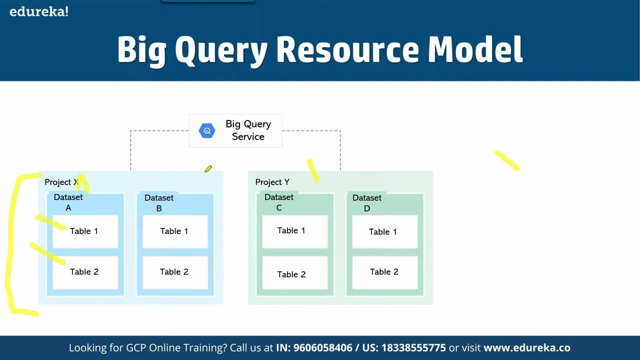 Now, this is a different project. Now, likewise, you can have different different projects here which can be integrated directly with your BQS, which is BigQuery service, wherein you can easily- you know- query the data. For example, this project needs some data with you know, this project or this project. 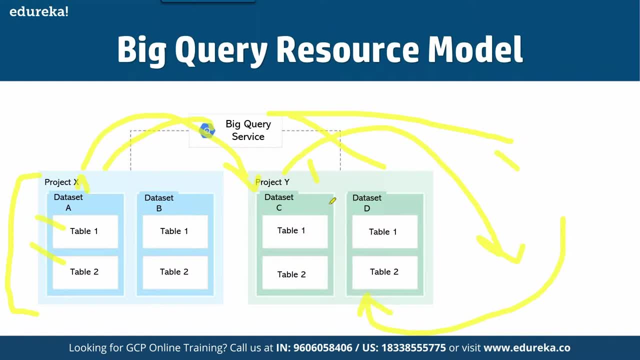 needs data with this project, or some different project needs data with this project. So this entire management, that role-based access control, can be easily be done with your BigQuery service. So that's again you know a little bit over here at a higher level. 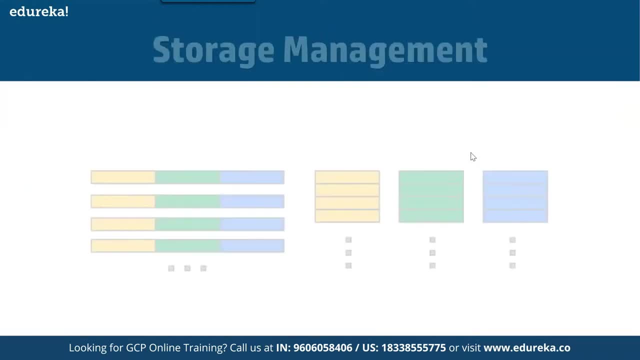 Now coming to the storage. Okay, So the storage management that we have. let's take a look at how storage management looks like of BigQuery and how it is different from others. So this is towards the left that you can see. this is traditional RDA BMS storage. 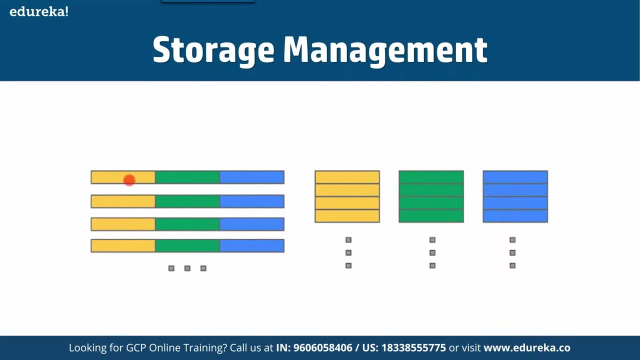 where you are going to have record-oriented storage, like this is the one record, second record, third record. likewise On the right side, you see this is BigQuery storage, So where it uses the column level storage. Now, even if I want to perform encryption, I can perform encryption in one column. 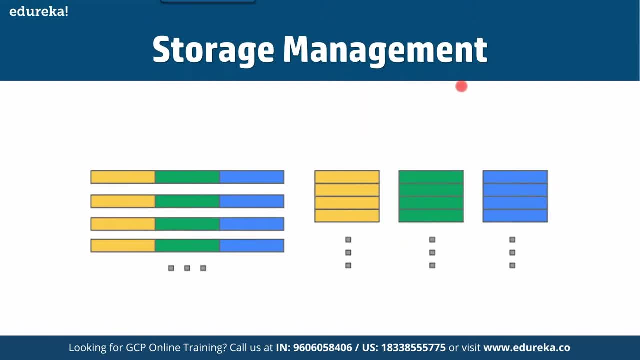 Maybe I have a data. let's say, you know, in one column I have name. second column I have their, you know last name. third column, I have their credit card number. Now this blue one is sensitive for me. 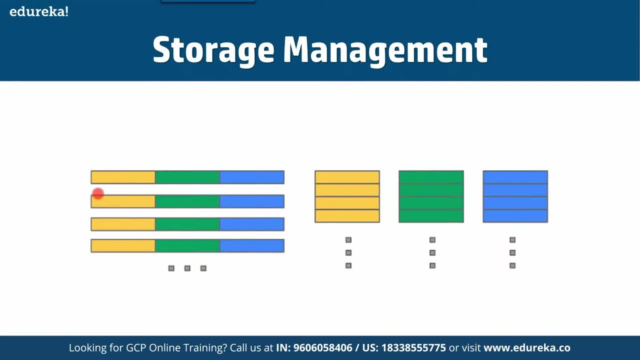 But if I go with the traditional RDA BMS storage, I have to basically encrypt the entire row. You know it's going to be difficult for me And at the same time encryption, decryption will take time. the operations execution will. 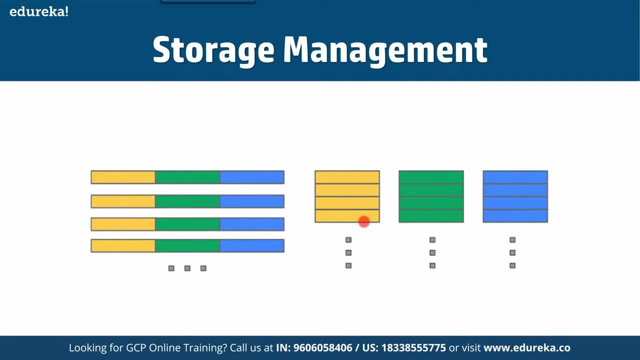 take time, which is going to be difficult. Now towards the right. if you talk about, you know, BigQuery storage. we are going to have the column level storage. We are going to encrypt one column at the time here. Now coming to the other one, which is storage management. 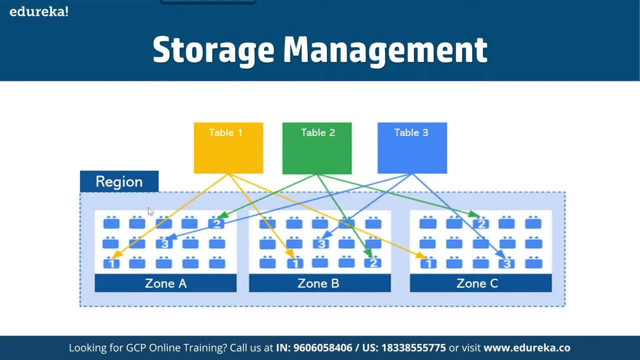 Now here, in this case, as you can see, like we have this table one, table two, table three In one region, we can have different zone, different zones, basically like your different data center. Maybe in India I have this data center in Bangalore, second is Hyderabad, third is Delhi. 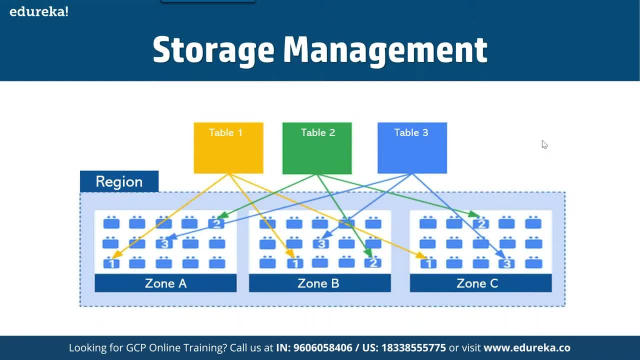 So if one zone is down, my data is still going to be there. at the second, at the third, Now here in this case, if you see, This second one is available here as well. It's available here as well. it's available here as well. 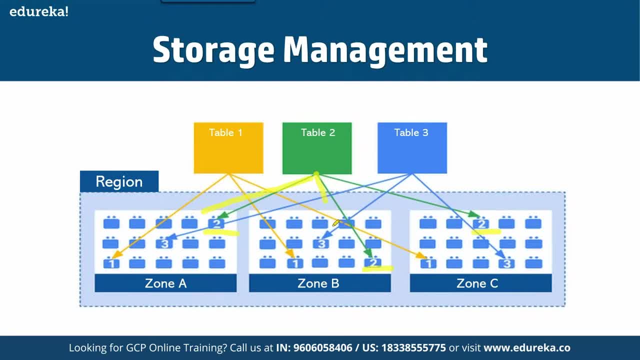 So the same data from table two is pointing out to this. The same data is copied at the second zone. same data is also copied at the third zone. So even and similar in this table one. this is copied in the first. this is copied here. 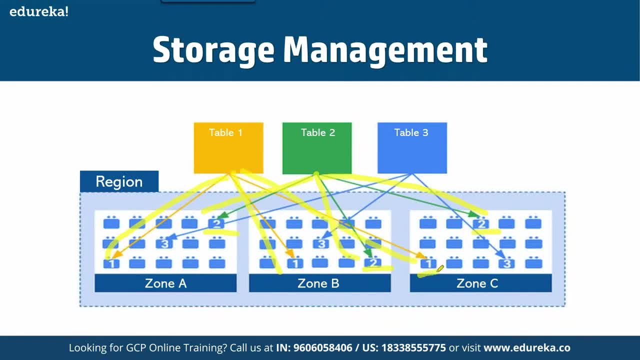 in the second. this is copied here in the third, which is this one, this one and this one. Now, in the third table, the same data you can see is copied here. It's copied here as well. It's copied here as well. 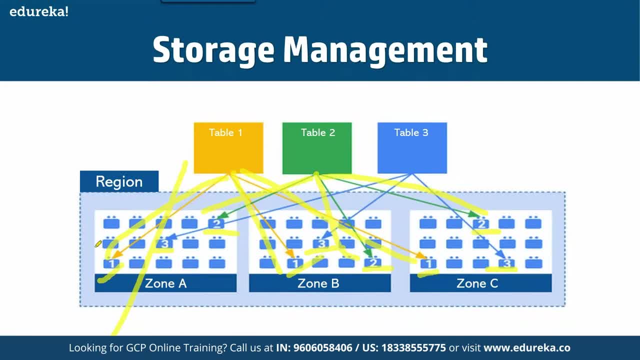 It's copied here as well. Now, if one, this one zone is going to go down, this is going to remain up. This is going to remain up. Let's say this one also got down. there was a network issue, So in that case, the third zone will remain up. 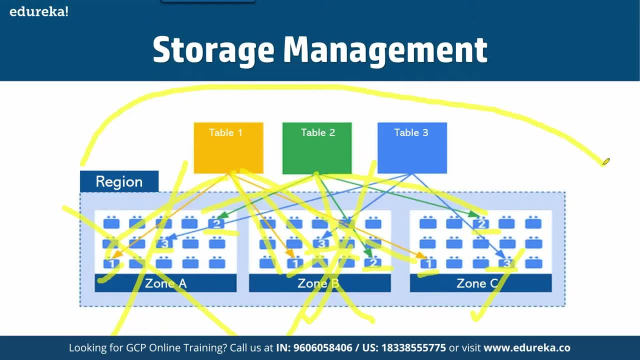 Now you can have multi regions as well, wherein the data from one region is going to be copied to the other region as well. So that's why it basically provides you a very good resiliency, and the data is going to be replicated automatically with the other data. 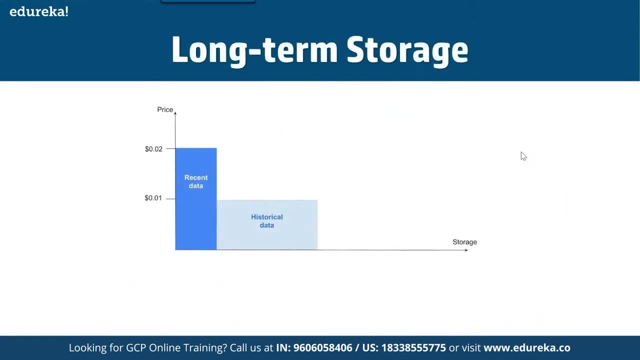 Okay, For the sake of ease. Now coming to LTS, which is long-term storage. So if you have a table or partition which is not modified for 90 consecutive days, it is considered as long-term storage and for pricing for the storage for that table automatically. 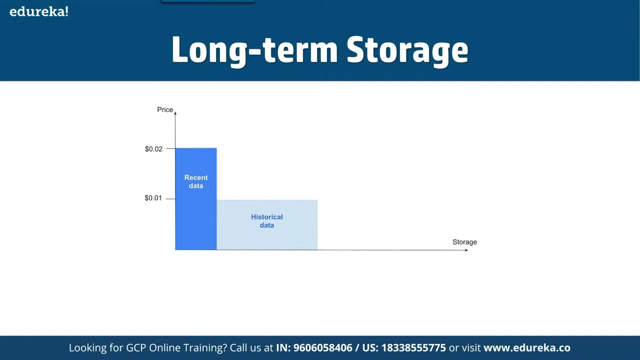 gets dropped by 50% to the same cost as cloud storage in airline. So basically, discount is going to be applied on per table, per partition basis. That's the biggest beauty of it. So if you're not using it, there is no need, there is no requirement that you have to change. 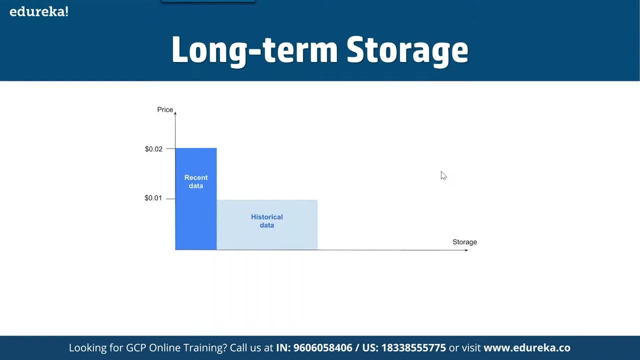 the storage type, It's automatically going to drop the price by 50% at the same cost. That's the biggest beauty of the Google cloud, if I were to say so, that you're not spending a lot of money on that. Moving on, what are different types of data ingestion that we have? 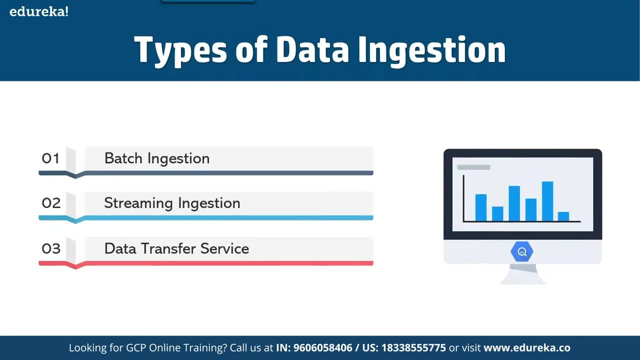 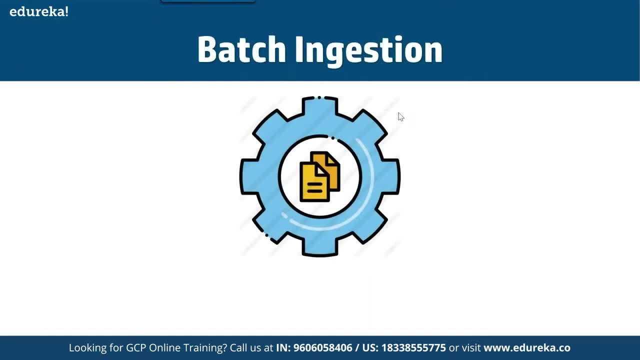 So we basically have a bad ingestion, We basically have streamlined, We basically have data transfer. Now let's talk about. you know Each of them one by one. What is the batch ingestion? So batch ingestion basically involves loading pages. you know basically having data set. 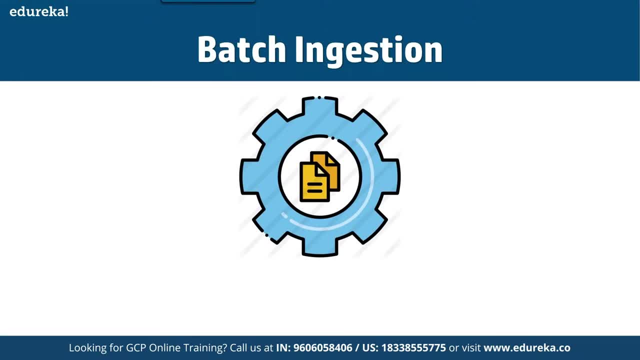 that does not have to be processed in the real time, So they are typically ingested at a specific regular frequencies and all the data which is going to arrive- It's going to arrive at one time or it's not going to arrive at all. 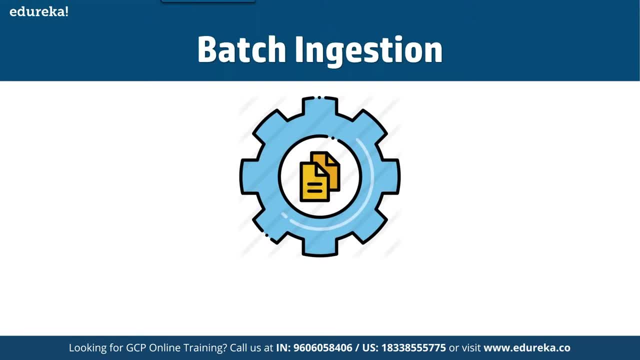 So the ingested data is then query for creating reports or combining with different sources where it can have data, So maybe different cloud providers. it can have data from your- you know- on-premise platform. It is going to be appeared together and at the same time it's going to be processed. 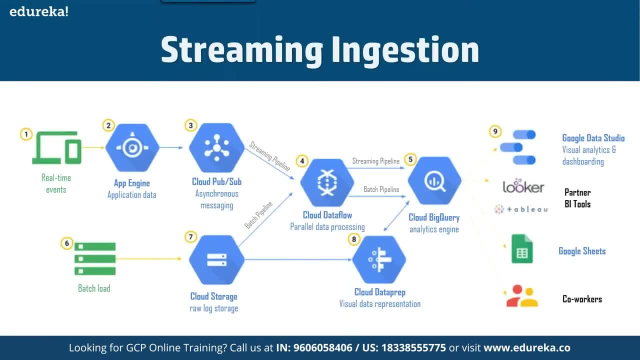 together In the case of streaming ingestion. it's a bit different. in the case of streaming ingestion- or you can see in this diagram- you know you are going to have your real time events. Maybe I have a service running so it's going to generate real time events. 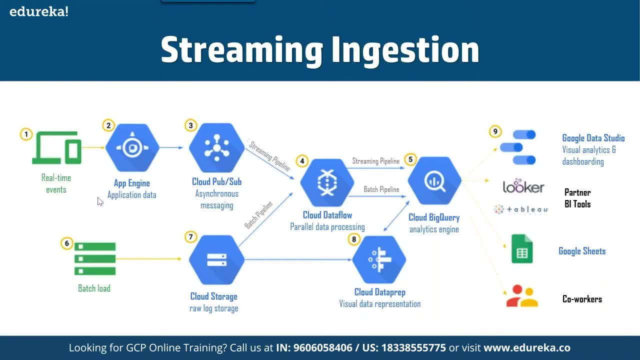 You are going to have, basically, the app engine which is going to be integrated with your applications, Can be on-premise, Can be on a Google cloud, Can be on, Can be on any other third party cloud as well, And these events are going to be, you know, fit together into your messaging service. 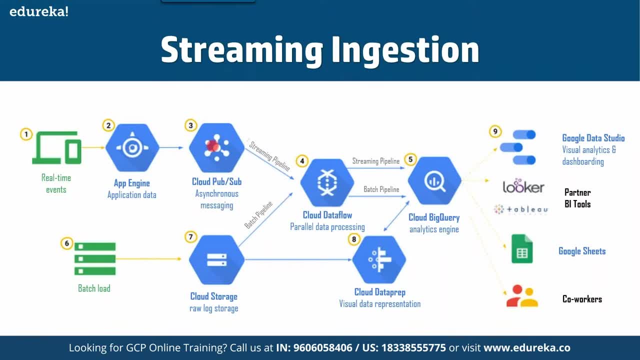 So any cloud model you talk about, for example your Azure, you have your Google or other- they provide the messaging services. So, different type of messaging services they are provided, with the help of which you can have the request response protocol set up, based on which you can also set the acknowledgement. 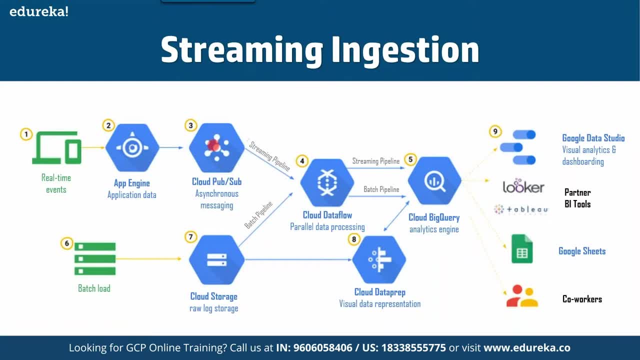 like the way TCP works. You send a request, wait for a response. If there is no response, you send another- You know- same request again, Because it will consider that your request has been dropped. So, with the help of stream pipeline, the request that you have received is going to be going. 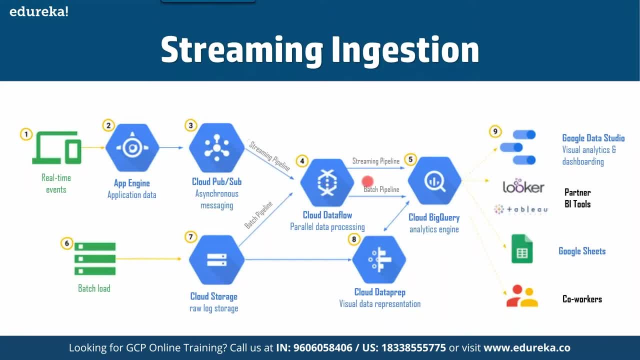 to the you know like, like a queue, where you can have multiple pipelines altogether, because it supports parallel communication, And next one, you have a batch pipeline where you can basically create the batch of CDs, batch of requests which is going to be, you know, accumulated in a queue together. 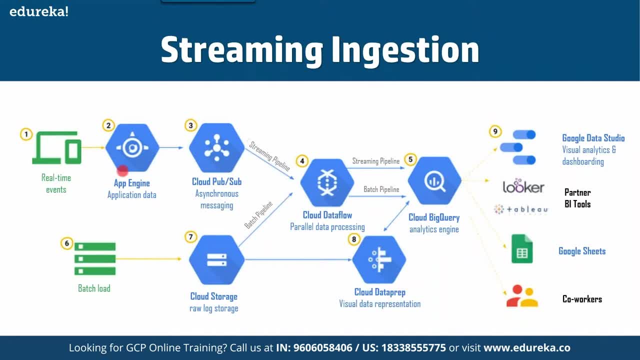 And at the end it's going to process together. Then after that you know you are going to have again. this is a batch processing data which is coming from. You have a batch load where the requests are accumulated and you know at a specific storage. 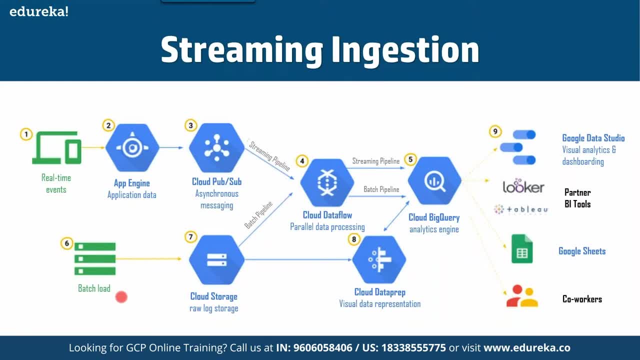 in the certain use cases, like your services are running maybe 2 pm every day, 3 pm every day, So it's going to, you know, ingest all the services from different sources to your environment at the same time, which is going to be processed by the cloud data flow and it's going to process. 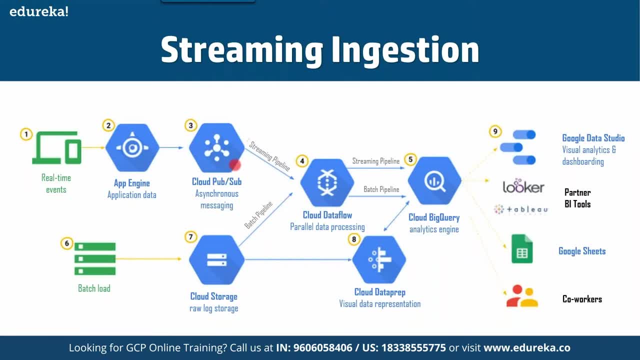 together. Again, this is a very big topic, guys. all three times We basically have a detail, even this in streaming and ingestion. We basically spend almost an hour on this. However, based on time constraint We have, That's why we're just talking about a bit overview of it. 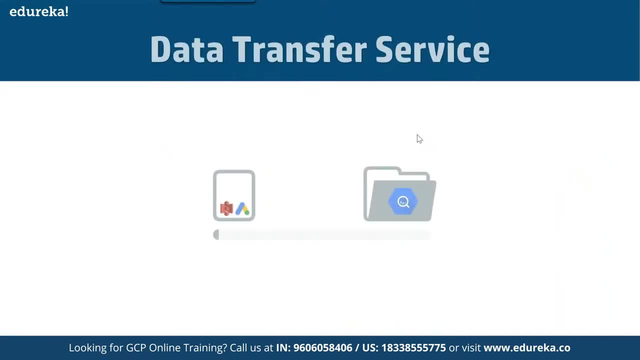 Otherwise, in general, this is a very big topic that we cover in detail. Now. the third service that we have is DTS, which is known as data transfer service. So you're you know, BigQuery data transfer service is basically a fully managed service. 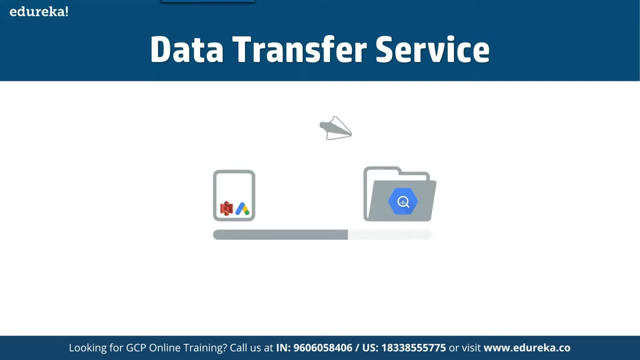 to ingest data from your Google SaaS applications as a software, as service applications, like your Google app, your external cloud service provider like Amazon, you know, and different, different providers we have, And You Can Transfer the data from data warehouse technologies like your data data, your Amazon Redshift. 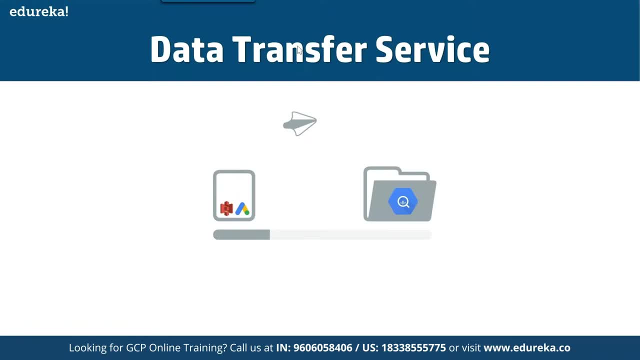 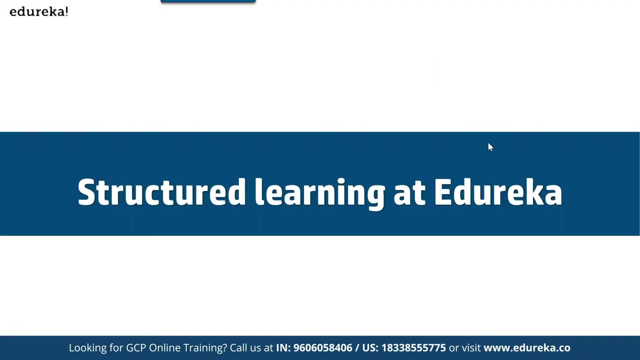 So all this thing basically falls into this category, which is data transfer service. Yeah, And out in this. Now coming on to the structured learning at Erica. So if you want to dive in more detail, you want to enroll for the course, and do you want? 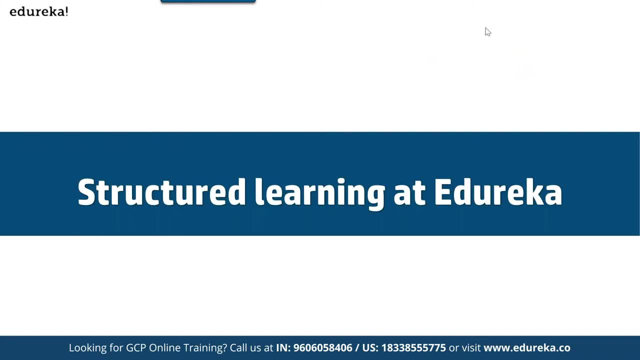 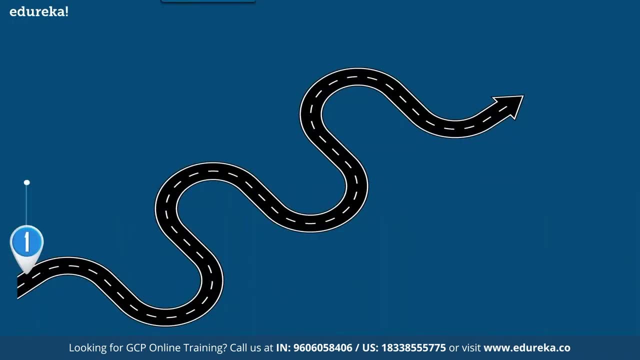 to know what the topics are. Like I said, we bring the transfer and see, so all this kind of topics. every information is available on our website, So let me just share The curve path, the learning path, how it's going to be there. 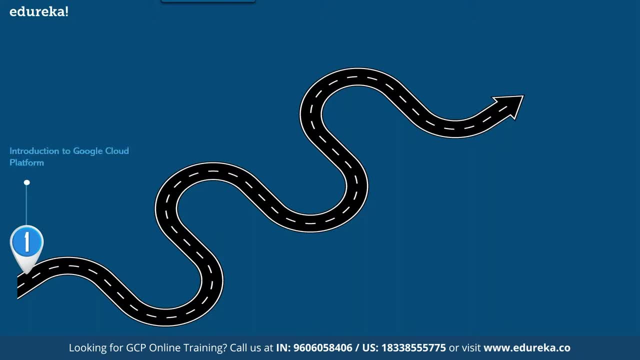 So, if you're going to enroll for the course, this is going to be the learning path. In the first class, you learn about Google cloud platform, how you can create your account, how you can set up the labs, its components, sub components, with the hands-on on different 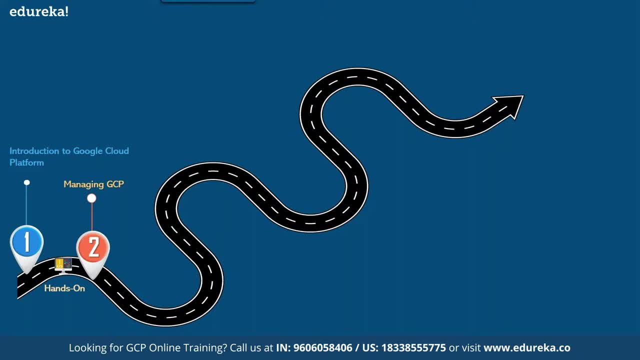 topics. Then after that, in the second class, you will learn about how you can basically manage your Google cloud platform, its services, its component and subcomponents, with the perspective hands-on. Then in the third class, you will learn about Google cloud platform, what's your networks? 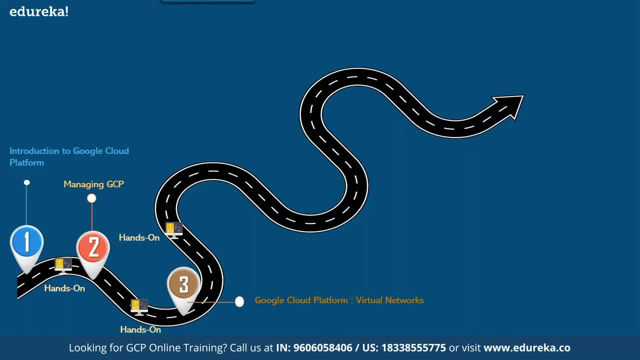 what's your different type of networks that you can create with the perspective hands-on. Then in the fourth class you will learn about security and identity fundamentals. You know how basically you can create different, different type of access You can, how basically you can control the entire access with you. 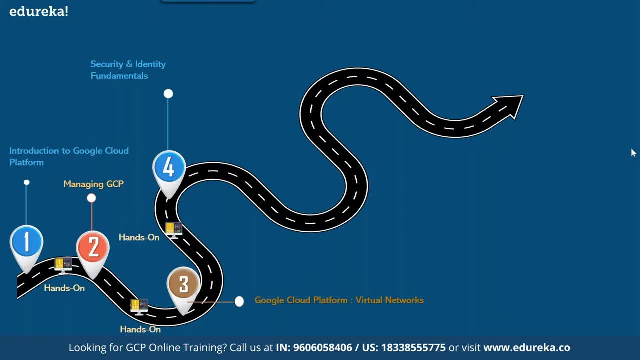 How, basically, you can give different permissions, how what are different roles that you can create? At the same time, you can also define your own structure, like how many roles you want, how many users you want. I don't want more than 15 users to access a resource. 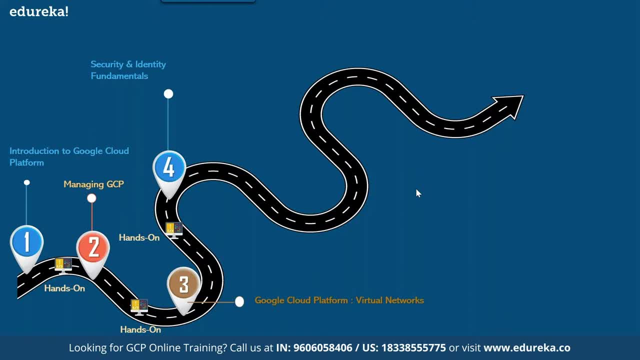 So all this kind of things can be restricted here- that we are going to learn with practicals, hands-on. Then after that you will learn about compute services, different type of storage that you have, different type of services that you can leverage, including the case of cloud. 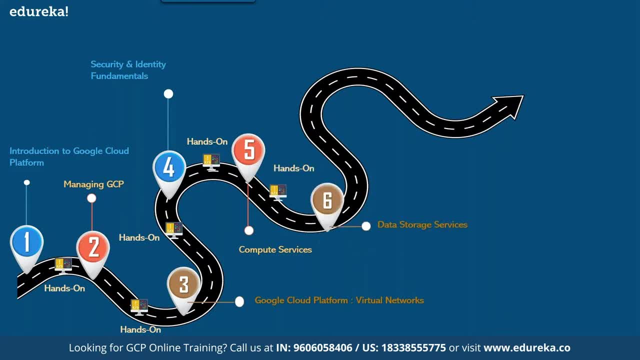 with the practical demonstration and the hands-on In the sixth class, you will learn about data storage services. What are different database that it supports, the different ways of storing it, What are the proprietary of you know Google? Google has provided you know various types. 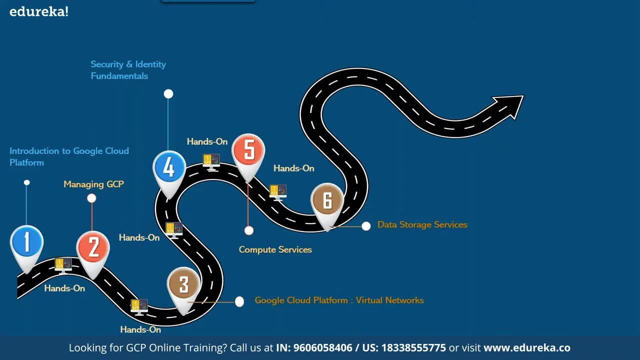 of different storage services which it's their own proprietary. What are they? What is the difference between them, How you can select which storage services based depending on the use case. with the practical hands-on, Then in the next class you will learn about architecting with Google Kubernetes engine. 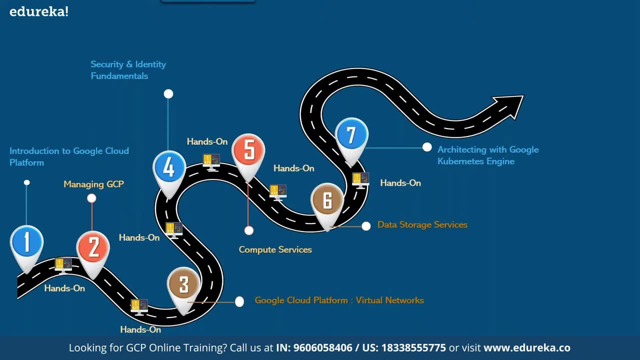 What is Docker? What is how you can integrate Kubernetes. you know how basically Kubernetes look like in GCP, How it is different from normal Kubernetes, How you can integrate with Docker Each and everything. you are going to learn in detail with the practical hands-on. 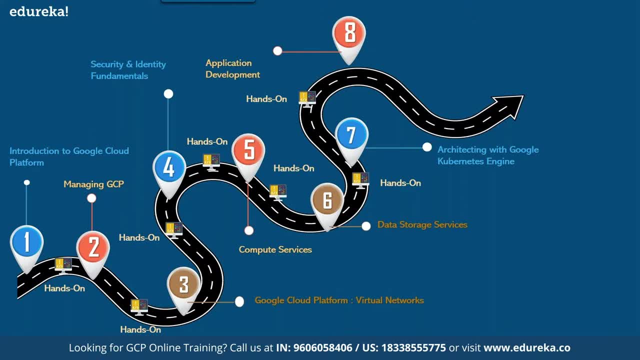 After that we are going to learn about in the eighth class, you will learn about application development. If you want to write the code, you want to develop the application, you know how you can do it. It's components of components, with the practical hands-on. 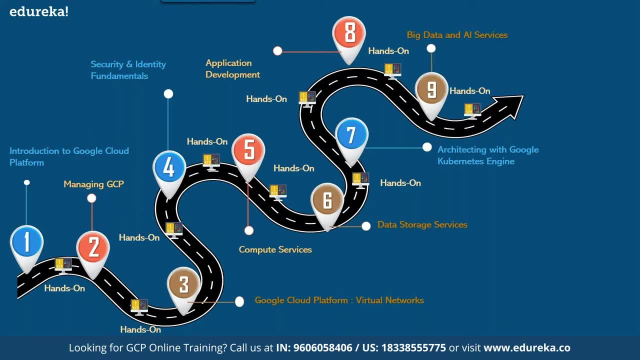 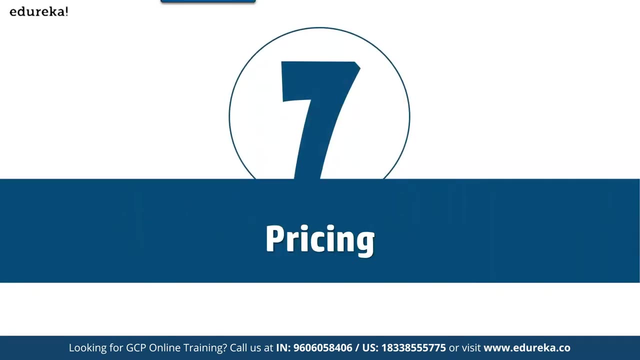 Then you will learn about big data and AI services with the practical hands-on And then, in the last class, you will learn how you can perform automation on the components with the practical hands-on. So this is the entire career path, I would say the training path for your certification, if you're applying to take 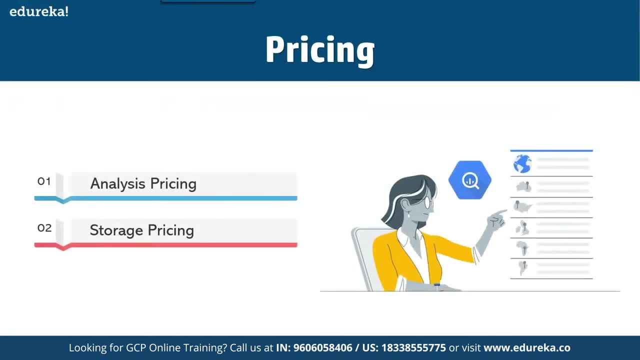 Now coming to the pricing if we talk about, we basically have two pricing model in the case of, you know, Google, that it provides. One is analysis pricing. Second is storage pricing. Now, if we talk about analysis pricing, this is basically on-demand pricing. 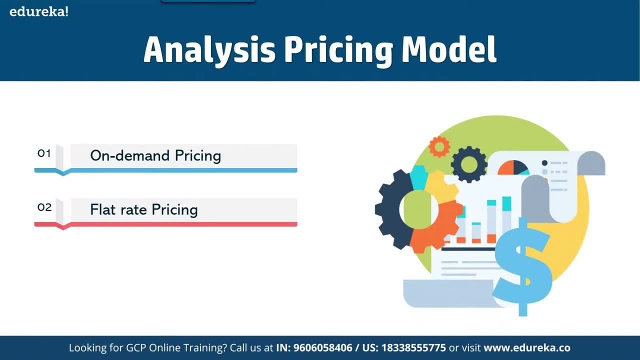 Basically it has flat rates pricing. in this We have three model. First is You are going to have the annual model. You are going to be basically billed and paid annually. Second is on a monthly basis. Third is basically the flexible store slots that you can choose. 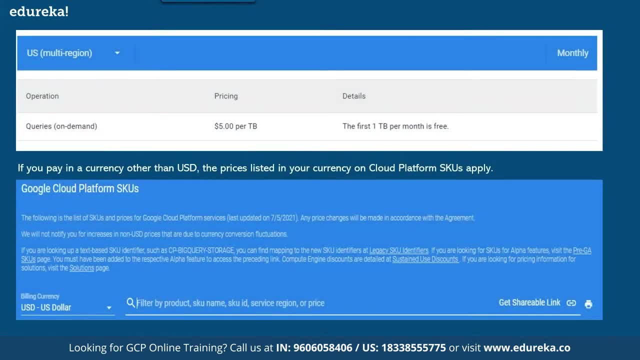 So this is again one of the example of the pricing model, the way it looks like. for example, queries on demand, you have to pay $5 per TB. So first TB is going to be free, but after that you have to pay $5 for every TB, which 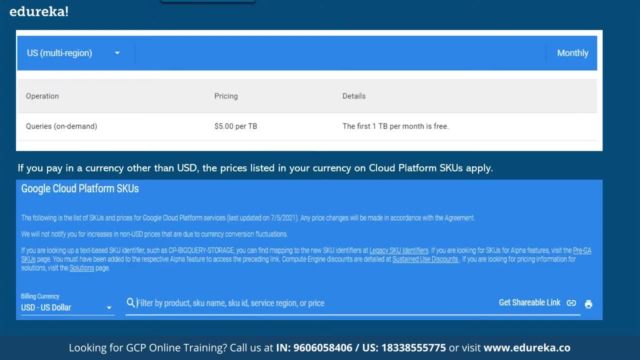 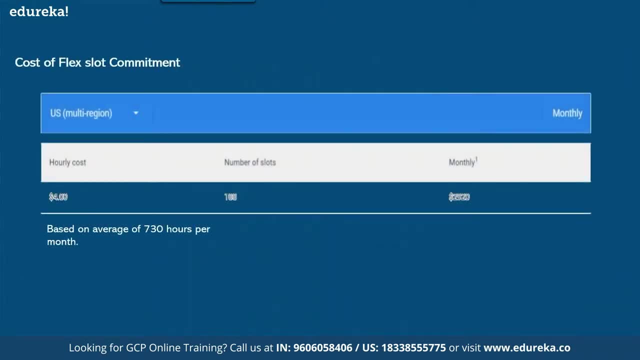 is a- you know a good deal as compared to other cloud vendor providers. Again, the same thing that I shared a moment ago: A different pricing model that it supports. Now, if we talk about the cost of a flexible slot commitment, like I said, we have three. 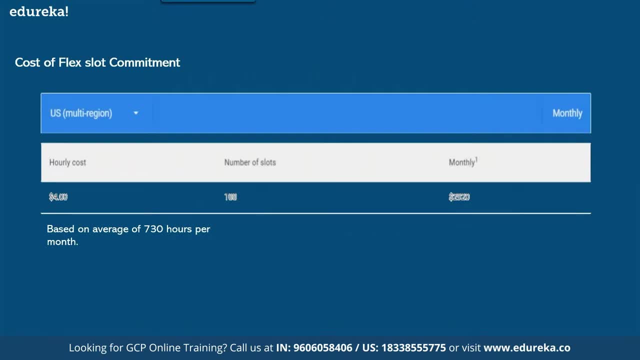 times the flexible monthly and the annual. So if you, if we basically take a look at flexible slot, you know you're going to get this much slots and you know, based on average of this is 730 hours per month, depending on your requirement. you can decide if you're using heavily. do you want to go with the? 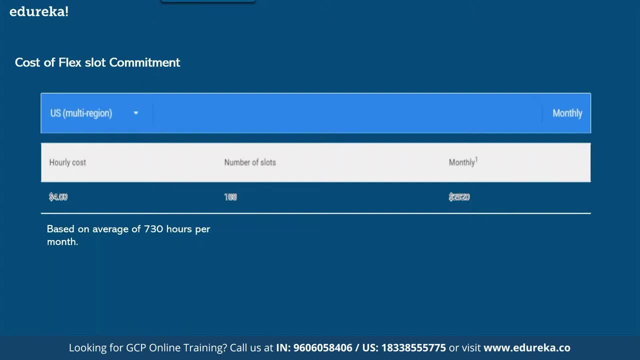 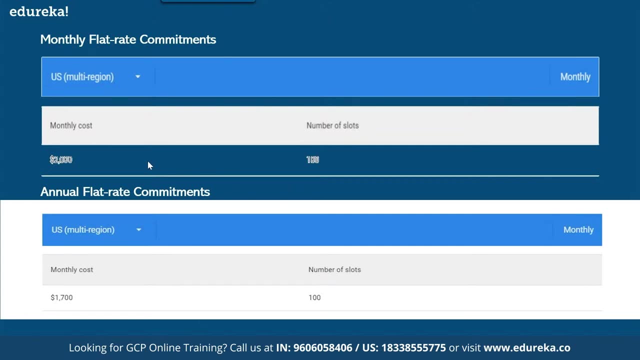 flexible, or your monthly is going to be best, or annually is going to be best Likewise. So in the case of monthly, the number of slots that you get is a hundred. You have to pay $2,000 for that. In the case of annually, the amount is less. 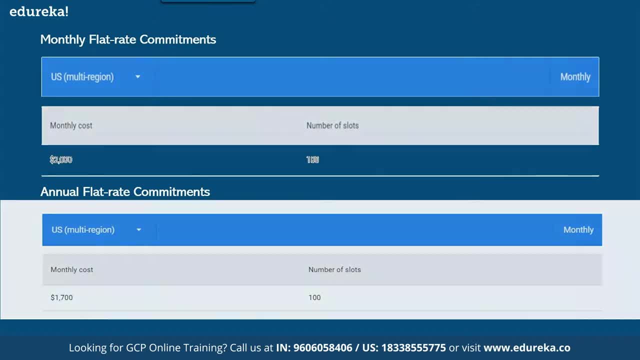 So where you're going to be less, which is $1,700.. Now, if you look at the cost in the case of flexi, it's a you know a bit more. now, basically, look at the cost of your monthly. it's high annually- is less, so you can save the money. 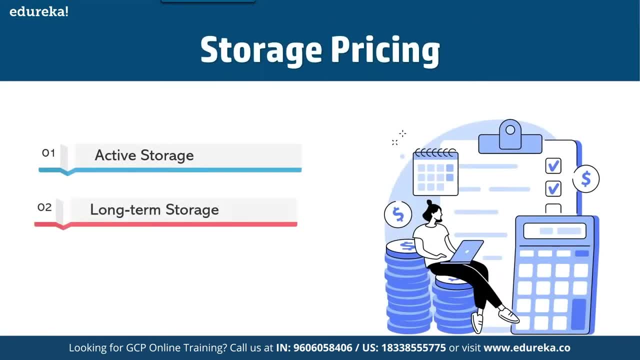 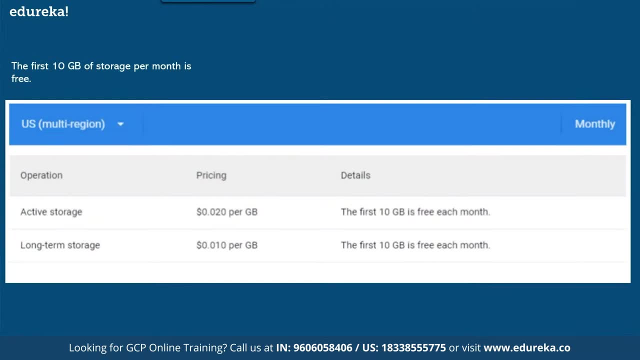 on that. Now, in terms of storage pricing, if you talk about, it has two types of storage pricing. One is active storage, Second is LTS, which is long term storage. So you have seen that, in the case of long-term storage, what will happen? that we even talked. 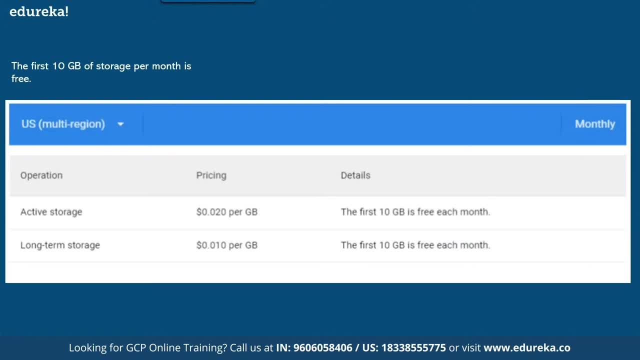 about a moment ago, which is which has a benefit that if your table or partition is not modified for 90 consecutive days, that is going to be considered as a long-term storage and price of that storage is going to be automatically dropped by 50%. 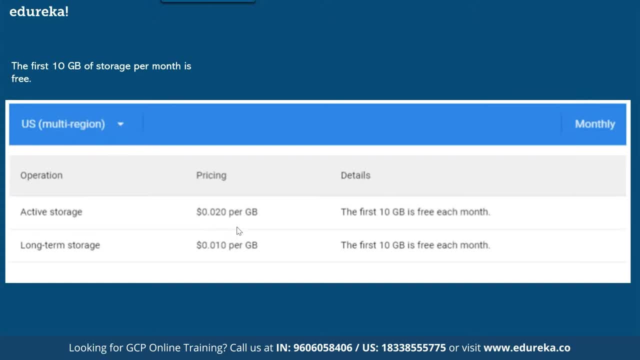 That's why, in this case, you see, for active storage it's the cost is $0.02,, 0.02.. And for long-term is 0.01, which is half, because the price gets dropped by 50%. And in both the cases- the first and GB are free. 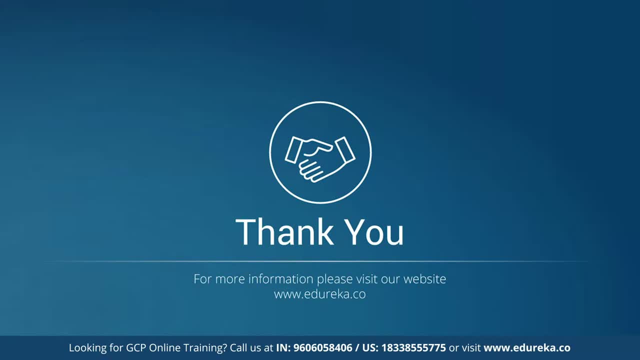 Okay, guys, if we can wrap up for today, it was an immense pleasure to meet all of you guys. Thanks for joining us today's session. Thank you and happy learning. Bye, Bye, Bye, Bye, Bye, Bye, Bye.